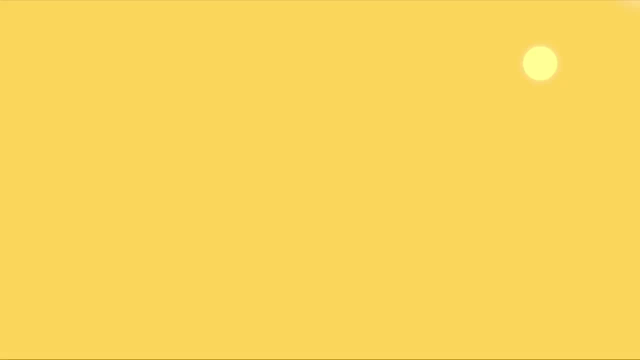 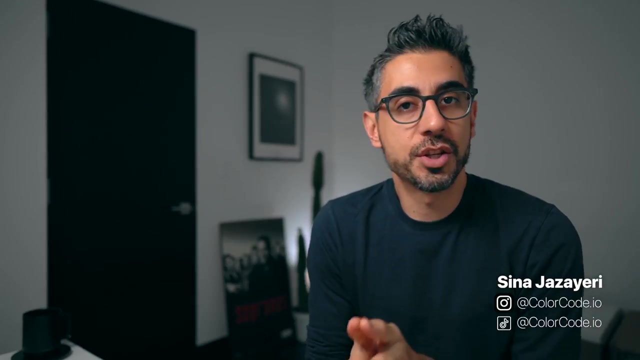 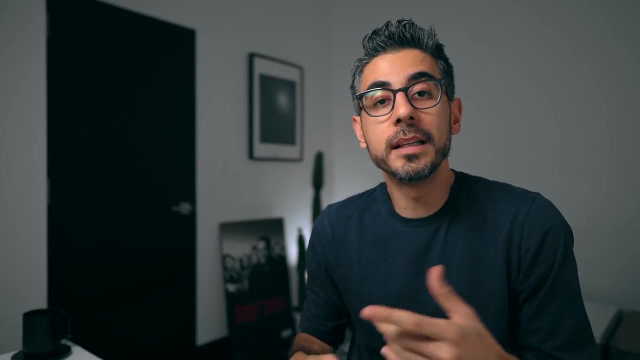 Let's go Higher order functions have been getting a lot of attention in the past few years because they're pretty heavily used in a lot of new patterns we've seen come to JavaScript, mainly thanks to functional programming And in no small part thanks to this guy, React. 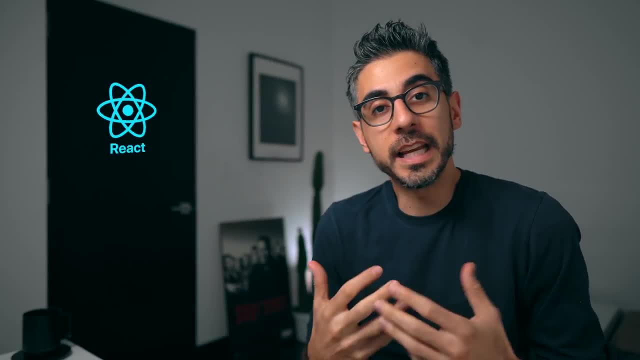 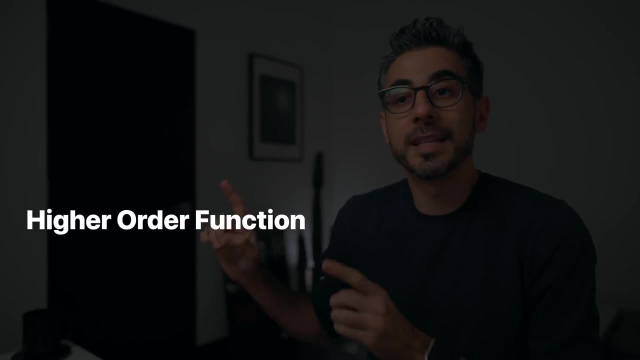 I see your React babies Now. React didn't really invent any of these patterns, It just really popped up and popularized them. So higher order functions, A higher order function is a function that accepts another function as a parameter or returns a function back to you. 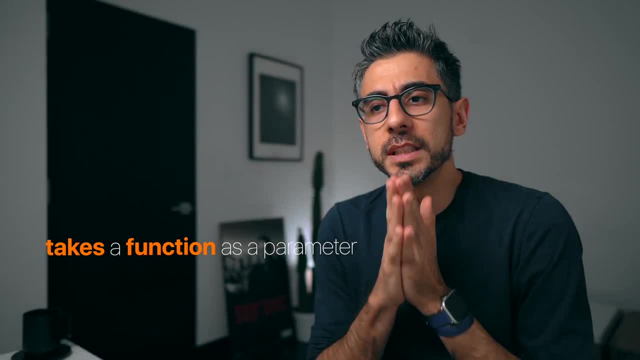 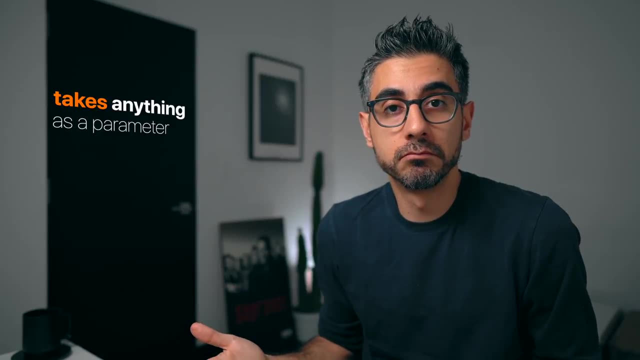 once it's done doing what it's supposed to do. Now, why would a function take another function as a parameter? Hmm, why would a function take any parameter at all? Hmm, what is the meaning of life? Well, a function takes a parameter. 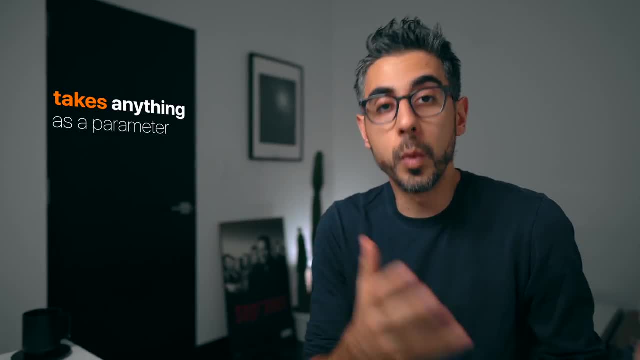 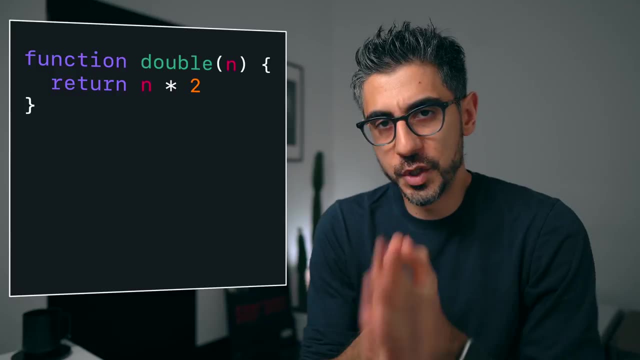 usually to perform some kind of operation on it or with it. Say a function that doubles any number you pass to it. I know contrived example and everybody uses this example. but just bear with me for a second. This function, this double function. 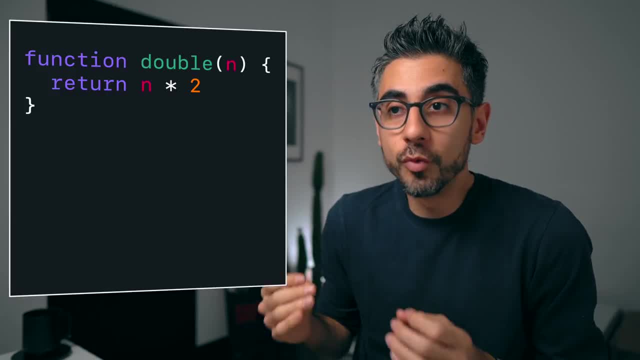 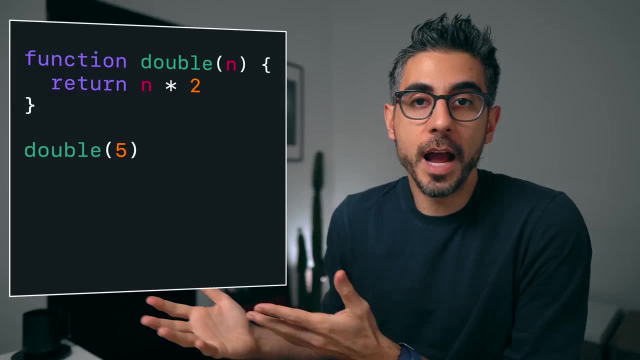 we call it double on its own doesn't do anything right. It really needs the incoming parameter in order to do what it's supposed to do, so it can double it. If I give it five, it gives me 10.. If I give it 40,, it gives me 80.. 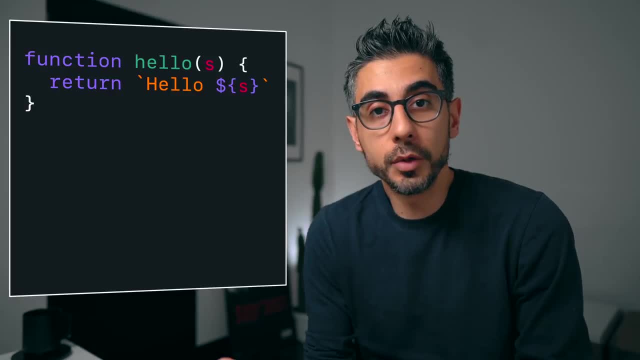 Or another function that takes your name and says hello to you, Or another function that takes your name and says hello to you, Or another function that takes your name and says hello to you. I pass it, Sina. it says hello Sina. 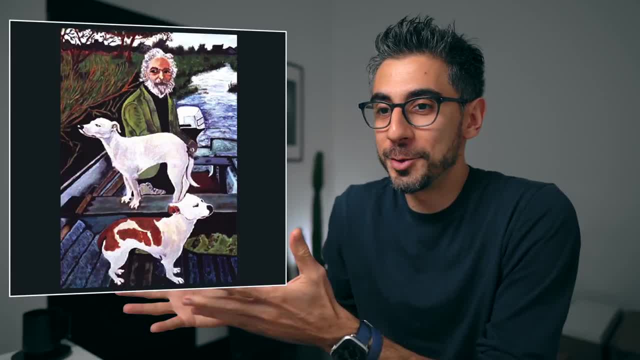 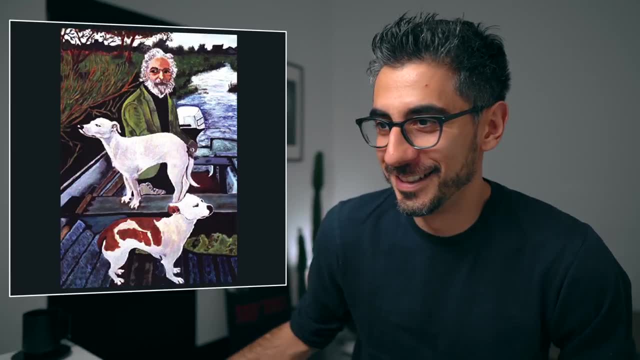 I pass it Oli. it says: hello Oli. One dog looks this way, the other dog looks the other way. Do you know what movie that's from? I'll give you a hint. Funny how, Anyway, both of these functions. 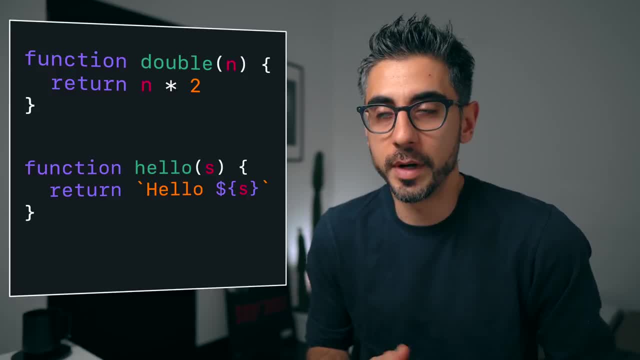 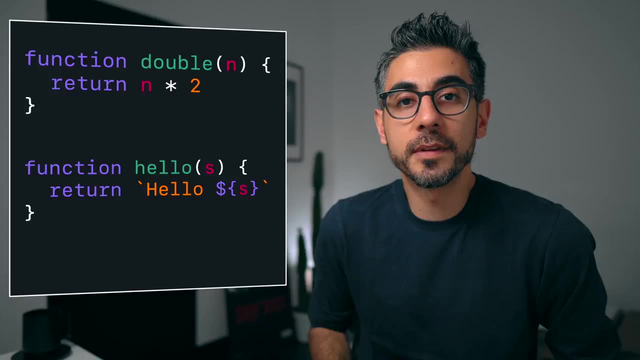 take a simple primitive type right: A number or a string, And that's all they need. Now what if a simple primitive value wasn't enough? What if your function had to do something a lot more complicated? Can you think of an example? 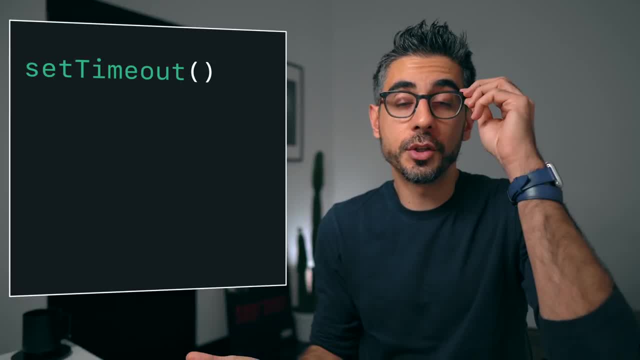 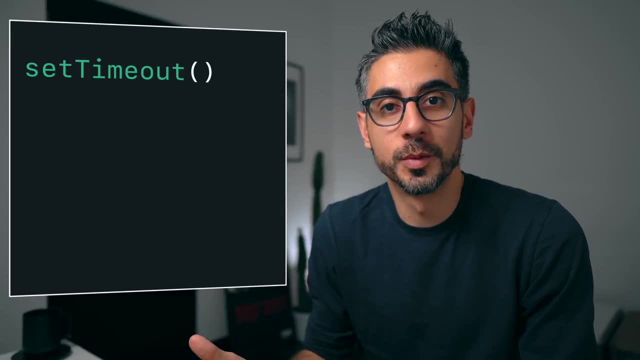 Well, how about setTimeout? I mean, what is setTimeout? That's just a function that waits a little bit and then it does a bunch of series of operations that you tell it to do. But how do you tell it what to do? You can't pass a number or a string, right? Telling setTimeout to do something is impossible to express using primitive values like a number or a string or a Boolean or whatnot. You need a function for that. Functions are a series of commands, and that's what makes them special. Here's a setTimeout API on MDN. 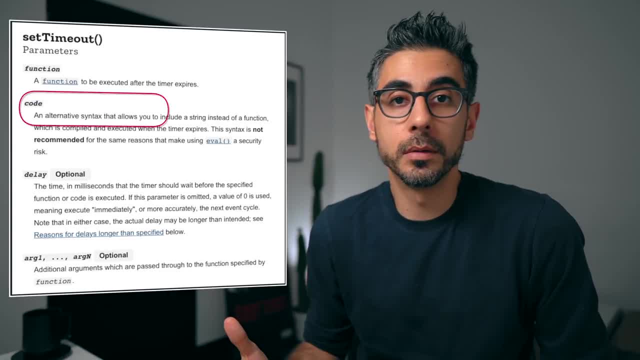 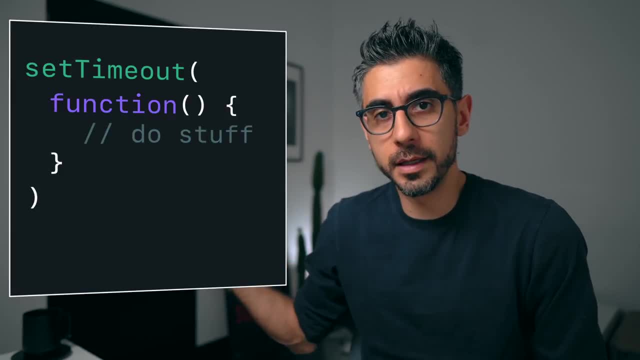 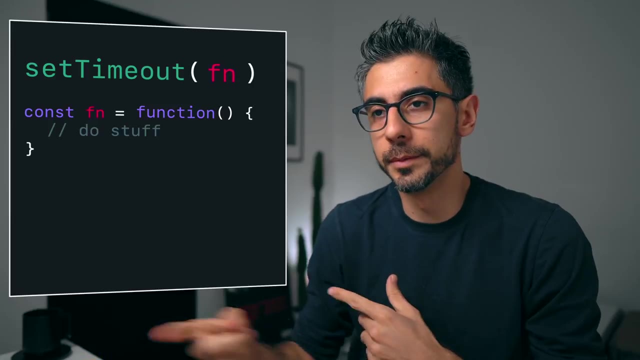 It takes a function- so what to do- and a number which is how long to wait before doing that thing. And just for reference, you can pass the function directly into it as an expression or you can store it inside a variable and pass the variable to it. 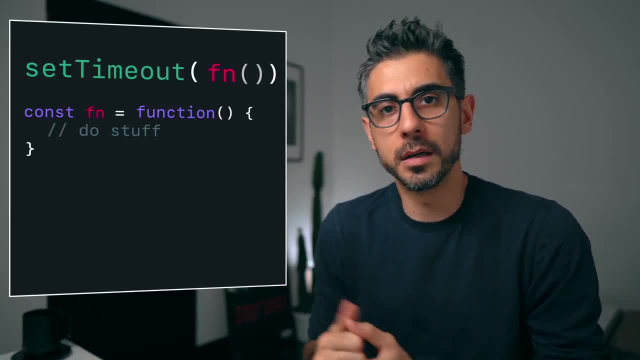 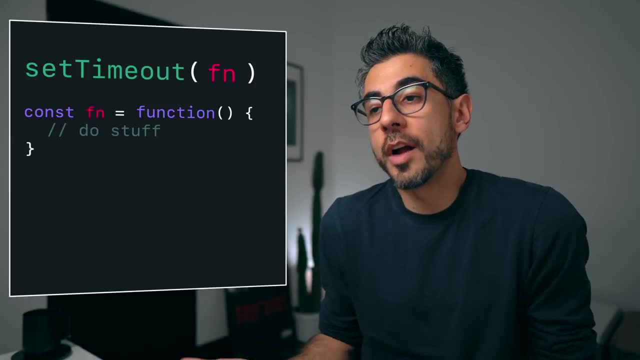 Just don't invoke the function when you pass it in, because then you are passing the return value of that function into setTimeout. You should know that. So now, what are some other higher order functions? Well, how about arrayfilter, In case you don't know how it works? 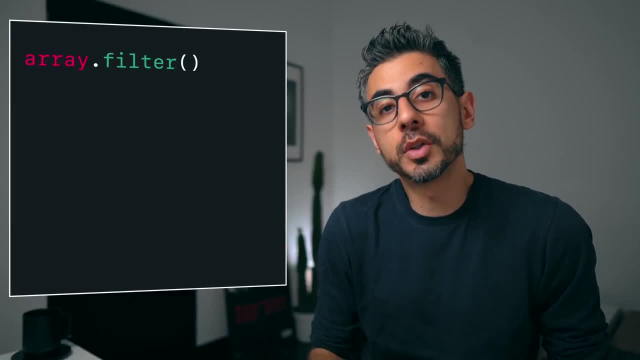 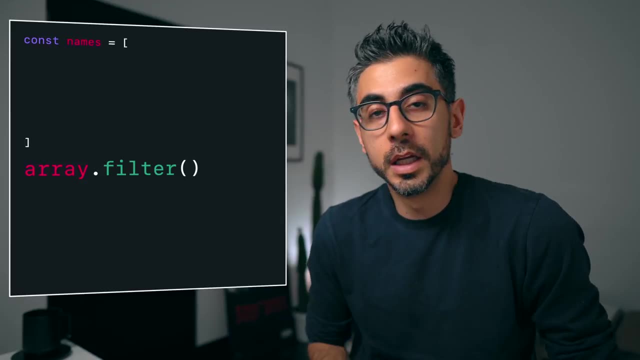 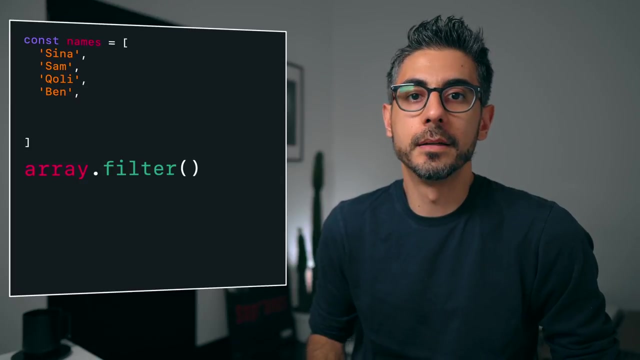 it's a function on the array prototype that helps you filter any array. So say, I have a array of names and I wanna filter out all the ones that start with a Q, because no name should ever start with a Q. So const names: Sina, Sam, Olly, Ben Zoe, Quinton and Alla. 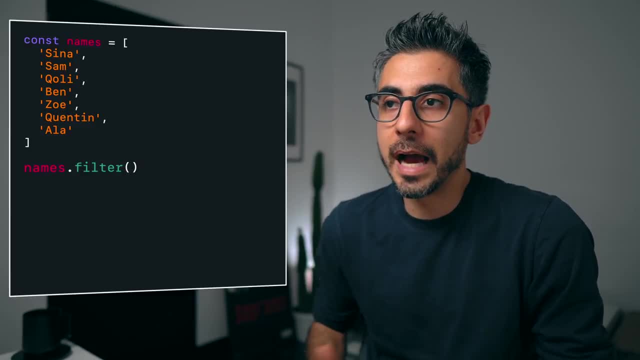 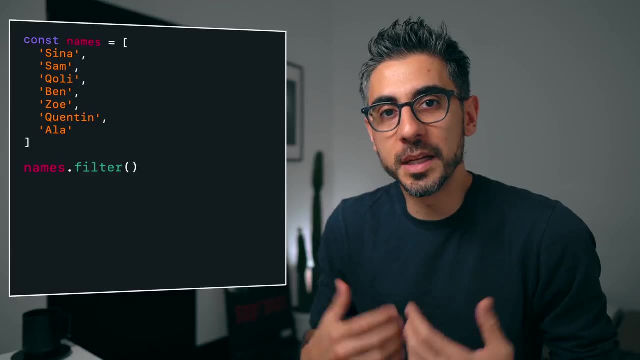 So I can say: arrayfilter- right, But how can I tell the filter function what my filtering logic is? Again, it's just impossible to express that using primitive values like strings and booleans. I'm gonna need to write some logic and a bunch of if statements. 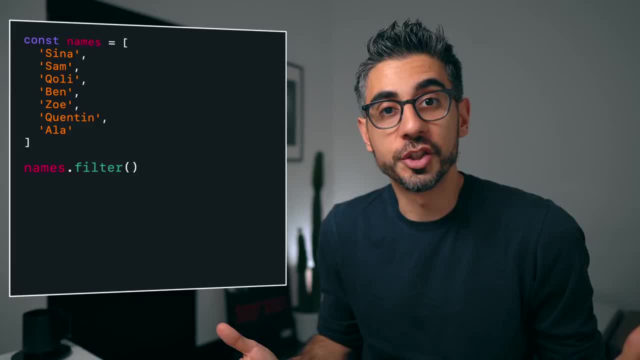 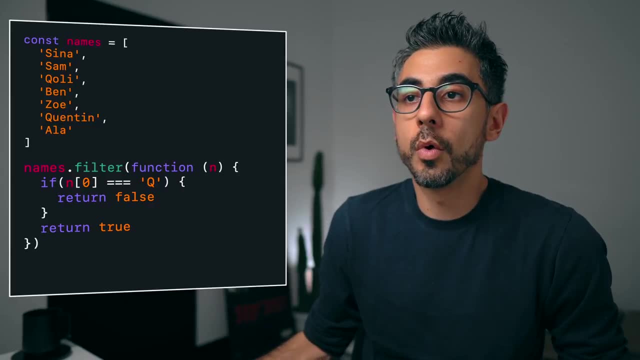 and all sorts of crazy stuff meaning a function. So in this case the logic is pretty simple: just an if statement and you turn false or true, Or you can use an arrow function and make it a little nicer and cleaner, because otherwise 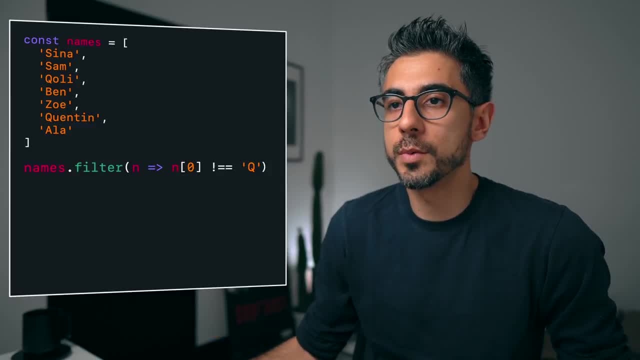 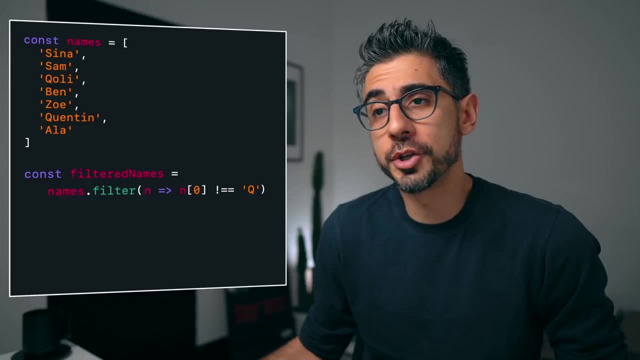 everyone's gonna yell at me in the comment section below. And of course, we can store the filtered list inside a variable and we can do what we wanna do with it. By the way, I covered arrow functions in the previous episode, episode seven. 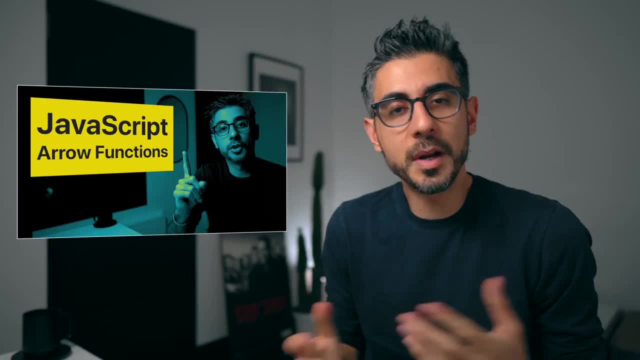 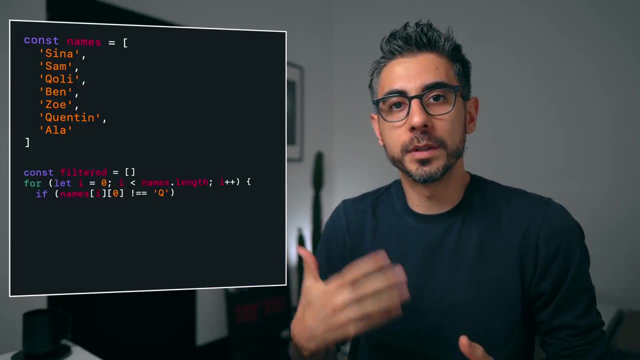 that's the one before this, So go check it out if you want. So now, why is this useful, right? Why can't I just filter the list the regular way, right? I can just iterate over the array using a for loop. 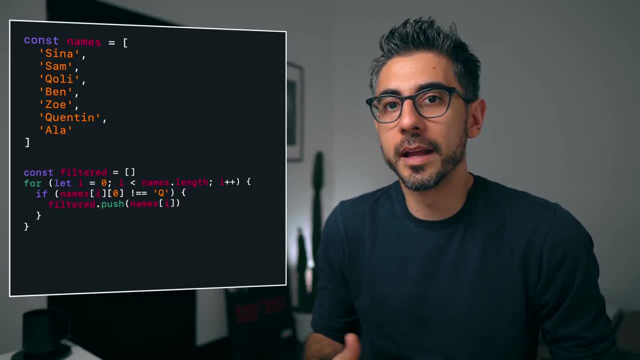 do the same logic in there: create a new filtered list and return it or store it inside a variable. Same results, right? What's the big deal with rayfilter? Why so serious? At first it may not seem like it's doing much for you. 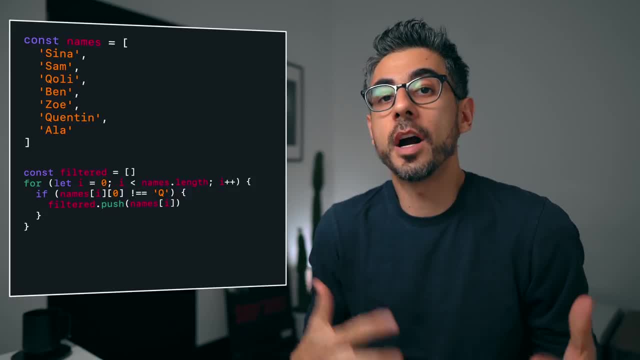 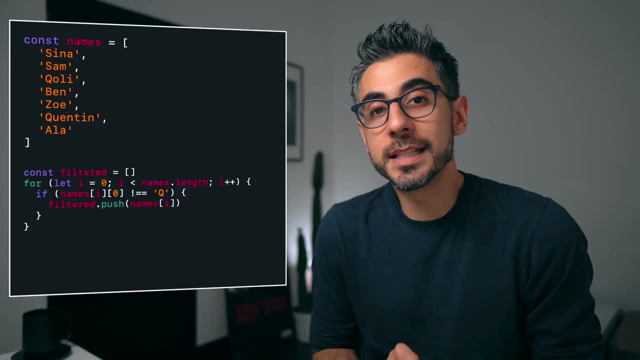 And if you think that I understand you, I come from a non-functional programming background and so for loops are very familiar to me, But filtering a list is a very common thing to do, So chances are you're gonna wanna do this more than once. 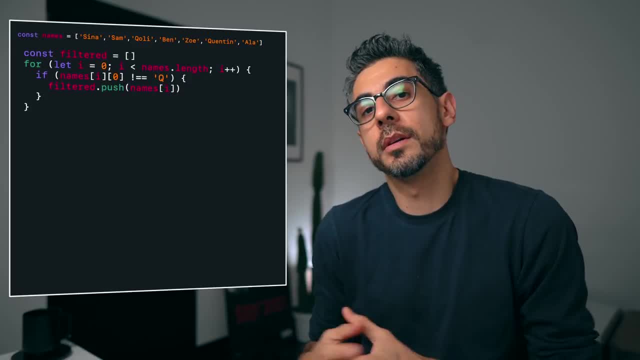 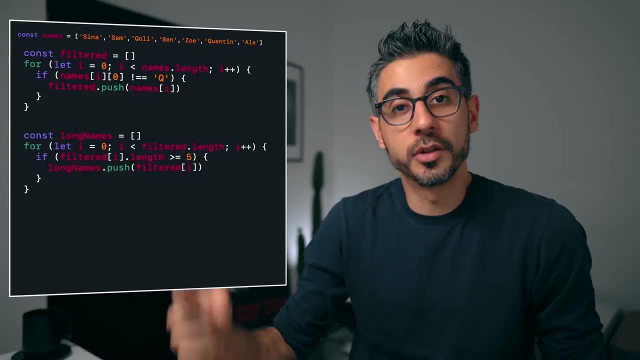 Maybe at first you're gonna want to do this more than once. You wanna filter the name starting with Q, Then maybe you wanna filter the ones that start with five characters or more, And then maybe you wanna then turn that list, that filtered list, into a list of DOM elements. 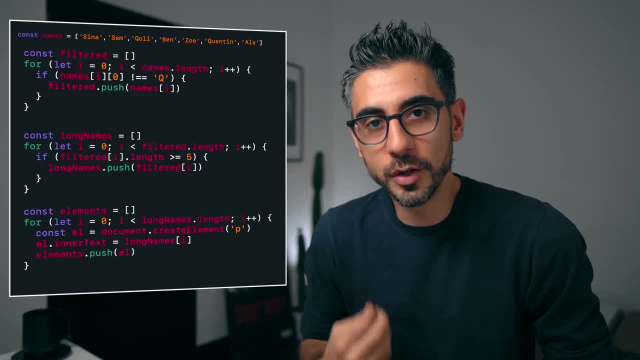 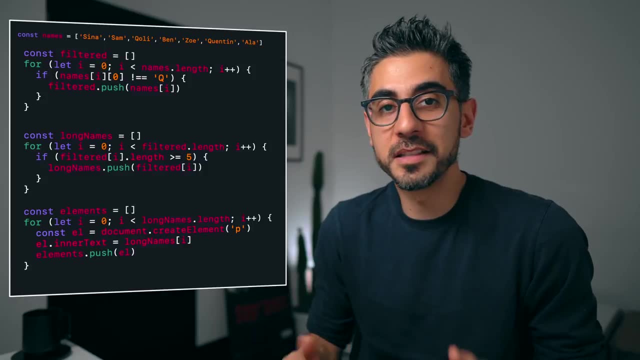 The point is, this is a very common thing to do, And you'll start to notice a pattern here, And the pattern is iterating over a list and creating a new list out of it. The only thing that's different between these three iterations is the actual logic on the inside itself. 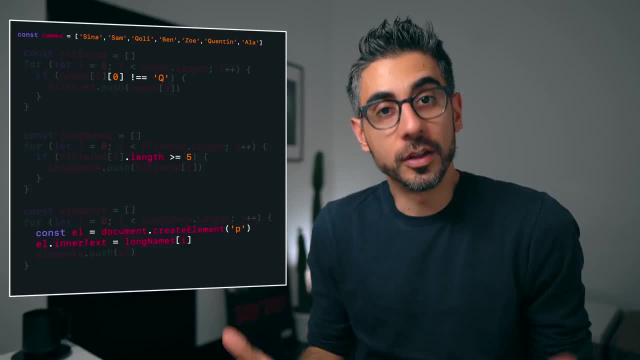 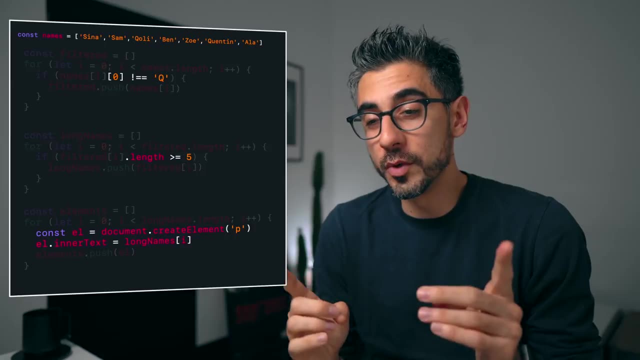 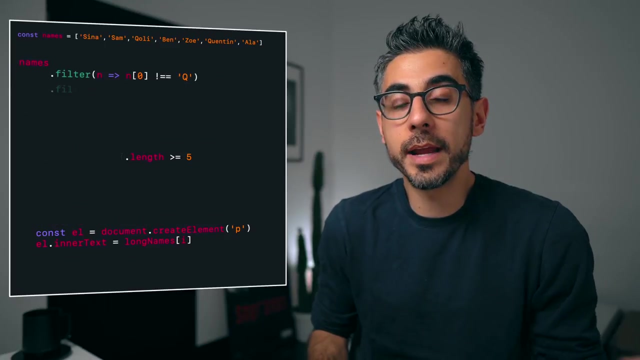 Or another way to look at it is that you're repeating a lot of these steps three times. Repetition is almost always a red flag, almost always. So using a higher order function in this case, you can abstract those repetitive steps away. 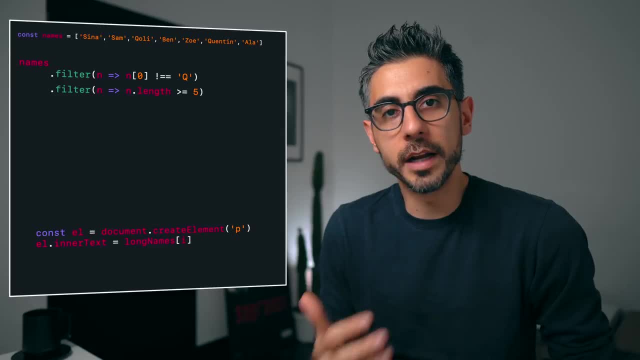 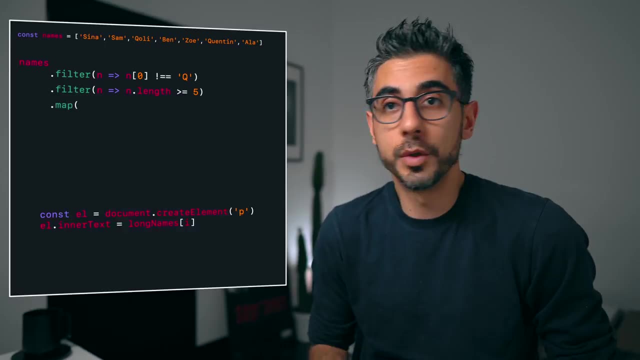 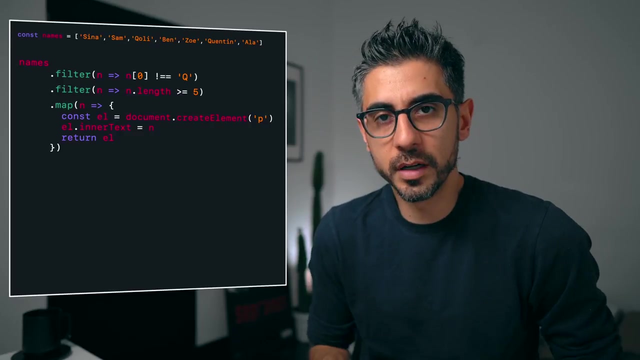 in this case using arrayfilter, and only worry about writing the filtering algorithm. So that's the real benefit here. Another example is arraymap. right, We use this in React all the time, Where you have an array of some data, maybe string or something. 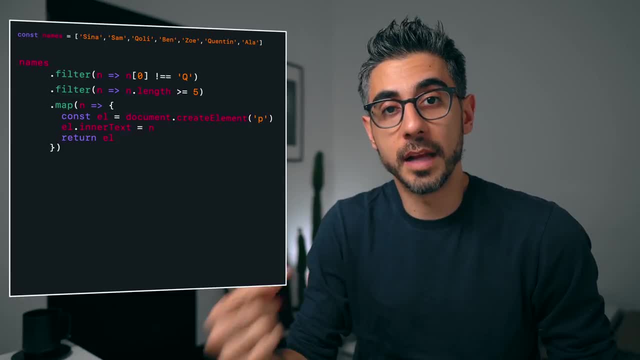 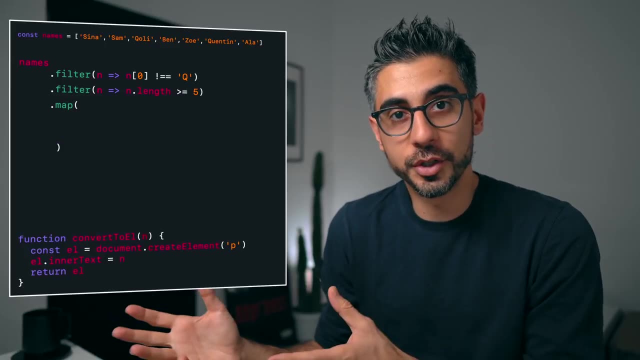 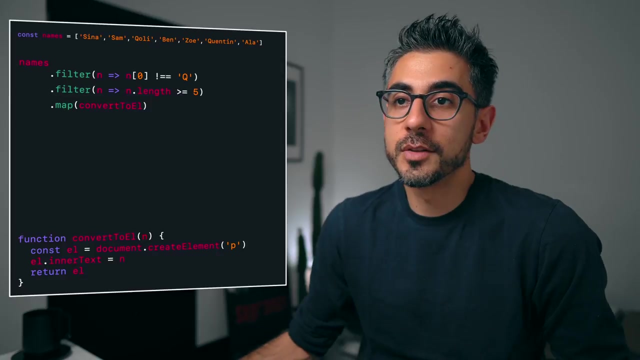 and you convert them into a list of JSX elements. So what ends up happening is you typically use a higher order function and combine it with these other functions, which we call first order functions. So any function that's not a higher order function, that's what we call them: a first order function. 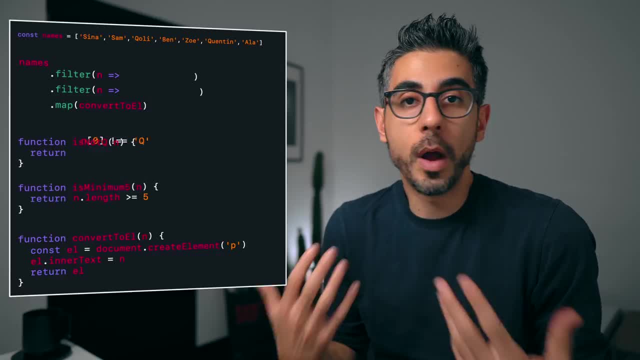 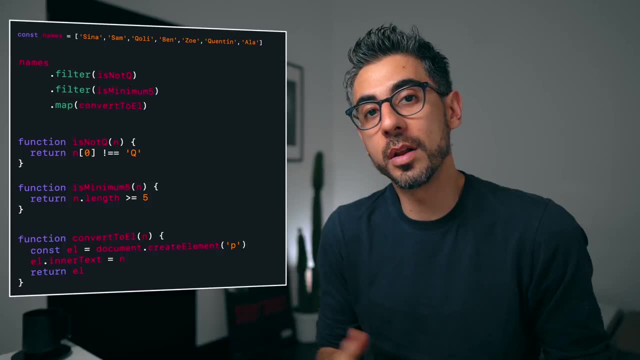 So this also means your functions are smaller, right? If you ever- God forbid- wanted to test your code, you should test your code. This makes it a lot easier, because now your functions are smaller and modularized. They do one thing, and one thing only. Without higher order functions, we wouldn't have arrayfilter or arraymap or arrayreduce, and that's a sad world. I'll also give you an example of one that returns a function. Remember higher order functions. the definition I gave you was that higher order functions. 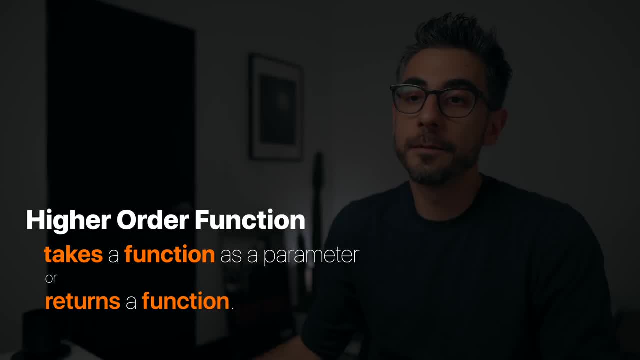 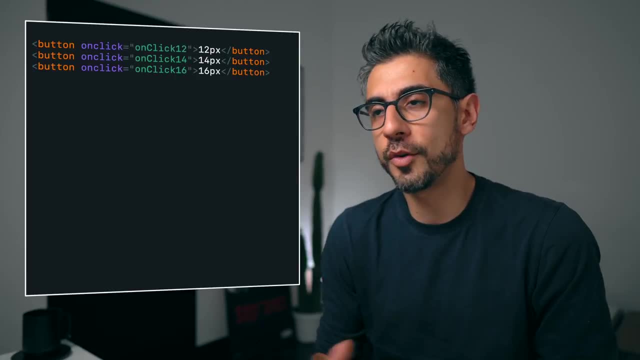 either take a parameter or they can also return a function. This is a pretty good practical example that's actually on MDN's page explaining closures of all things- the topic of next episode, by the way, episode nine. So say you have three buttons on the page. 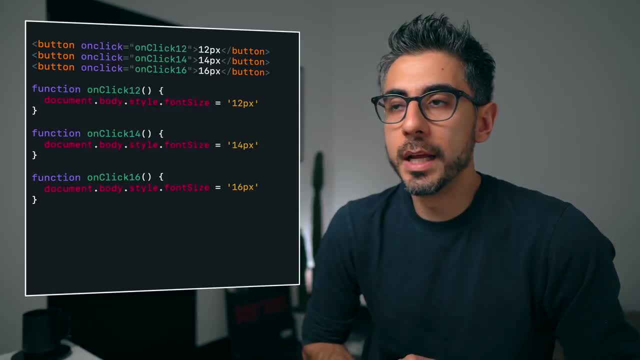 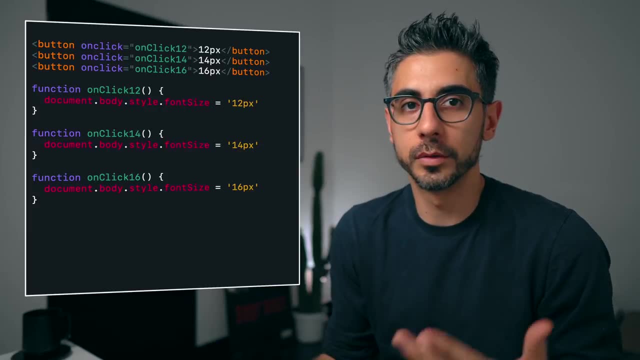 and all they do is the same thing, but slightly differently. Like they all change the font size of the page to 12,, 14, or 16,, depending on who was called, who was clicked, Instead of writing this logic three times. 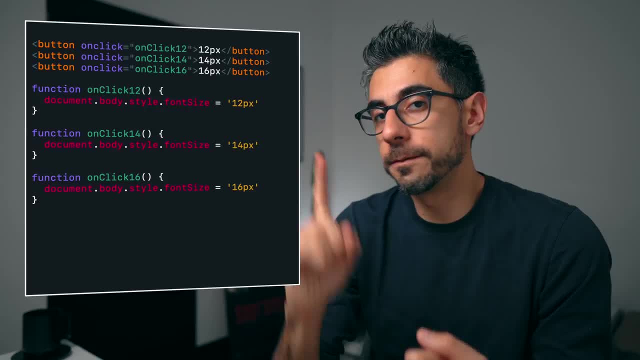 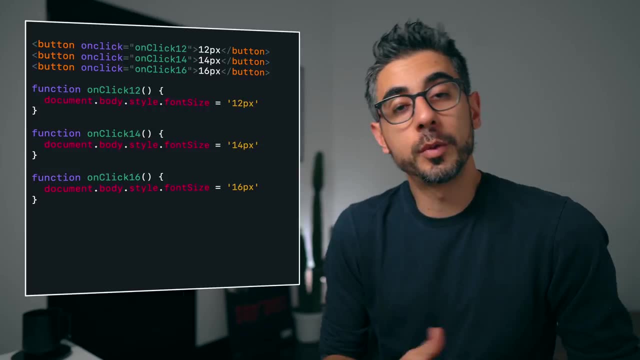 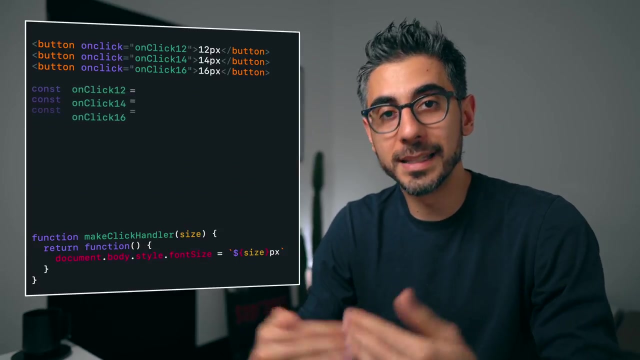 like that. you abstract away the logic that includes finding the body tag and changing the CSS value of the font size to whatever it is, And you create a function factory that generates and returns functions that then will be used as click handlers for each of those buttons. 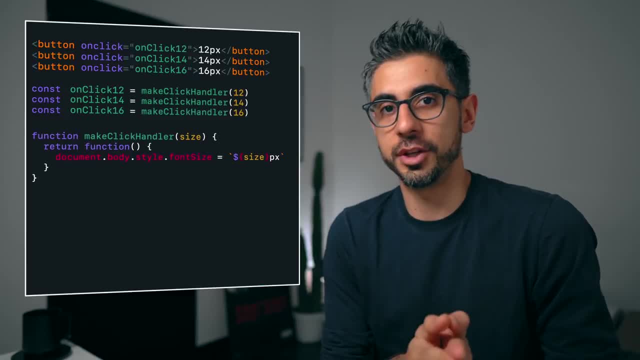 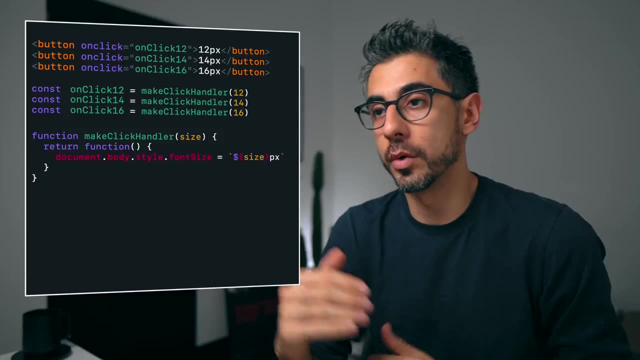 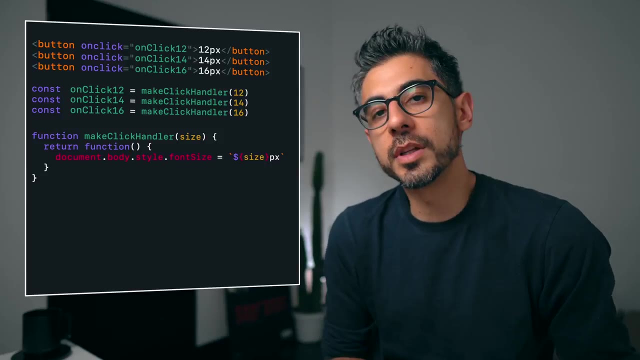 By the way, function factory is not to be confused with factory functions, two totally different things. This way you write the logic one time inside your, your higher order function and you take a parameter based on which button is calling it. So each button essentially gets a copy of that function. 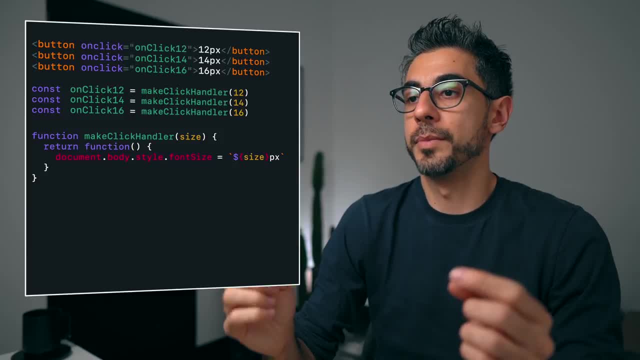 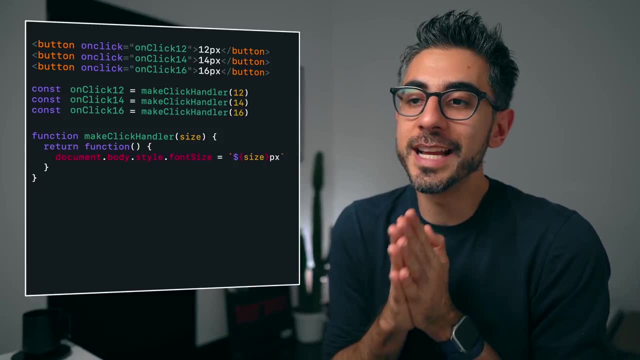 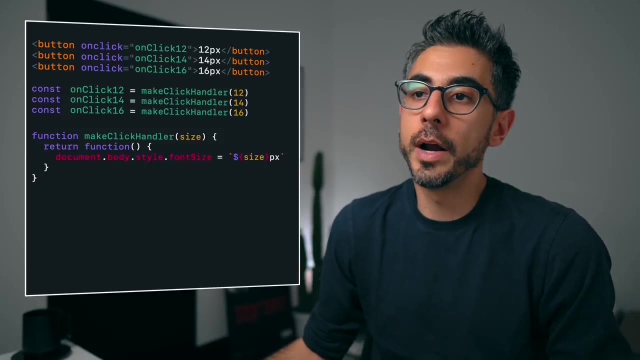 that was created inside the higher order function with their own specific font size logic baked into the logic itself. That function factory is an example of a higher order function that returns a function back to you and hopefully you see the utility of it All right, this was a shorter episode. 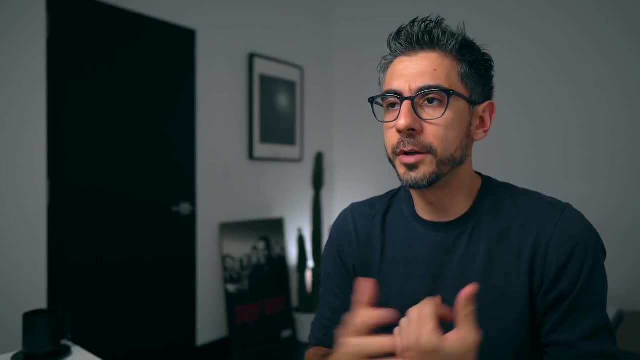 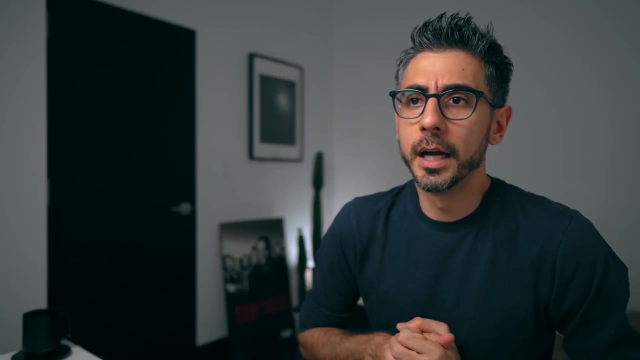 but one of my favorite topics to talk about And I didn't do any live coding today and this time I'm testing this new format, but hopefully it made sense. Hopefully you like that. Let me know in the comments if you have an example of a higher order function. 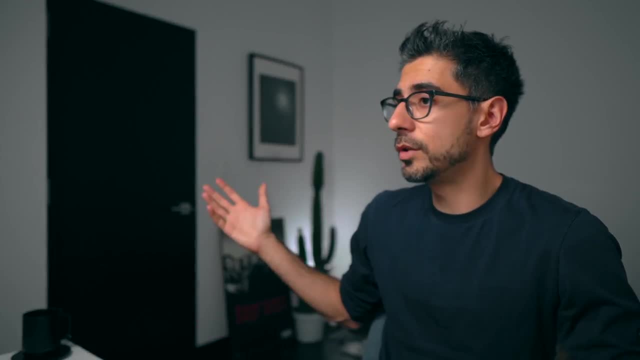 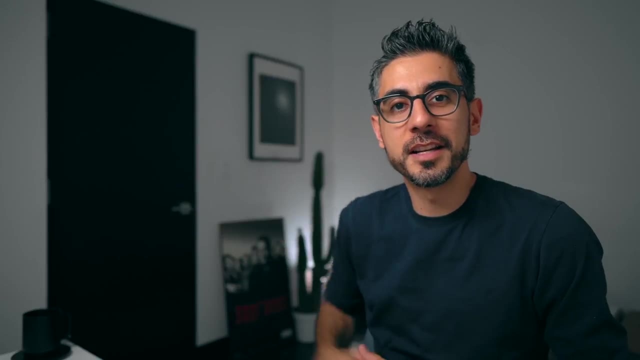 that you've run into recently. let me know what you think about this new format and what you think about my new studio. I have moved and I will no longer be able to see New York City on the outside using my windows. I'm in a closed box right now, but yeah. 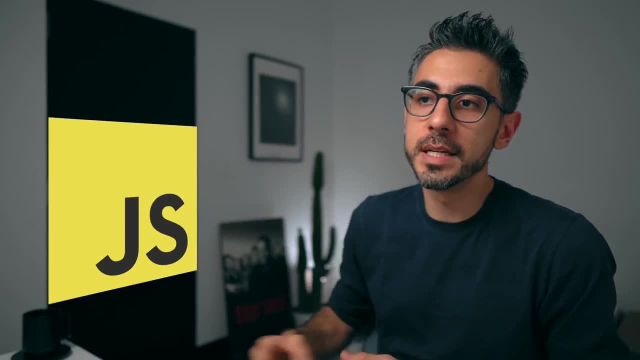 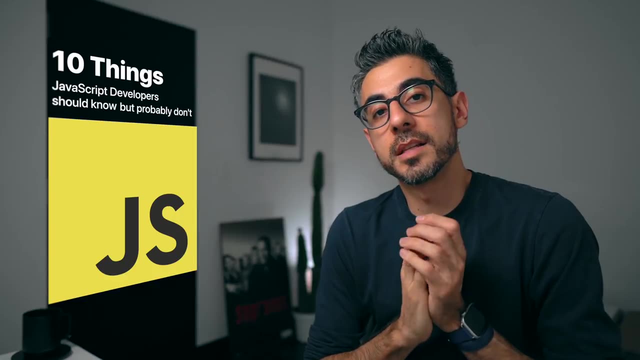 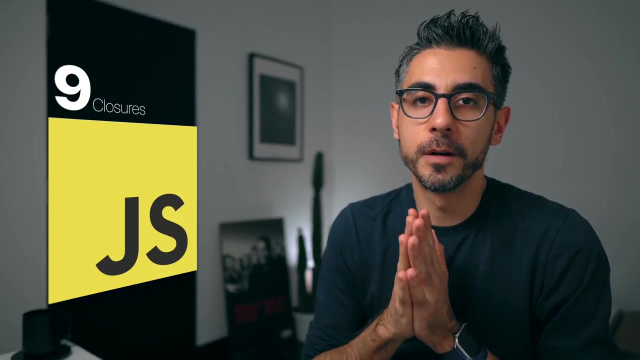 thanks for watching. This was episode eight of this 10 part series. I'm calling 10 things JavaScript developers should know but probably don't. And, as I mentioned, the next episode, episode nine, will be dedicated to closures, an amazing, amazing feature of JavaScript. 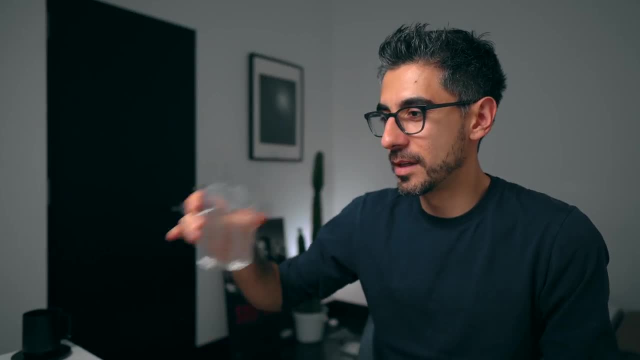 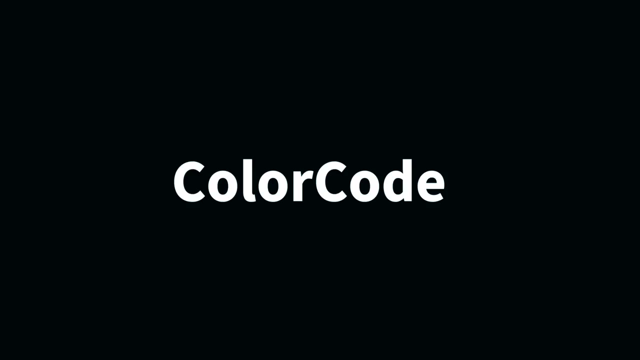 Hope to see you there. Salute.